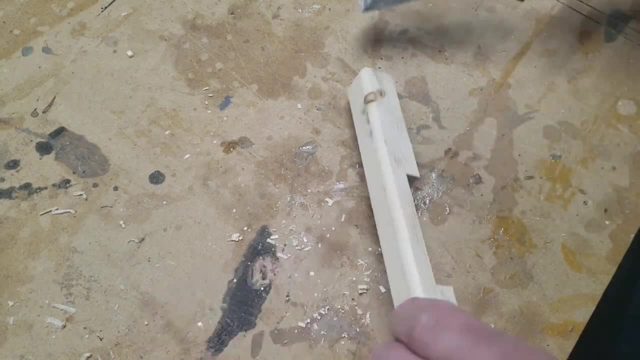 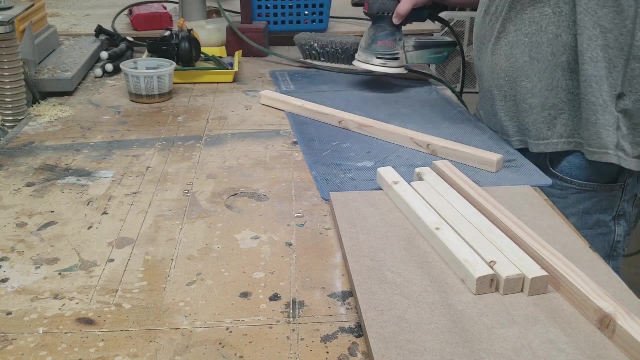 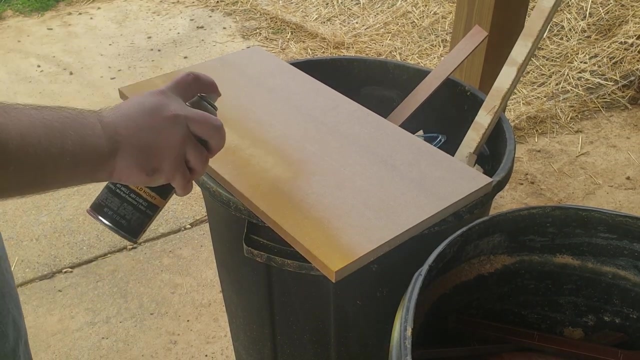 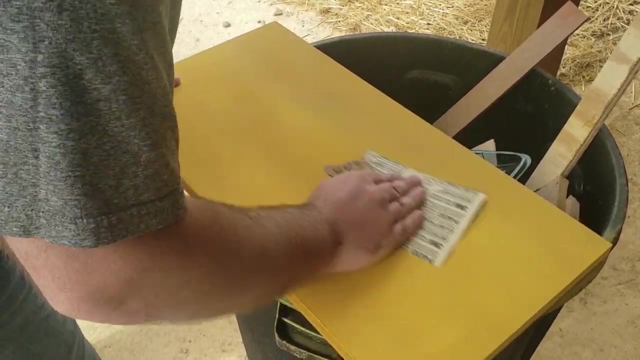 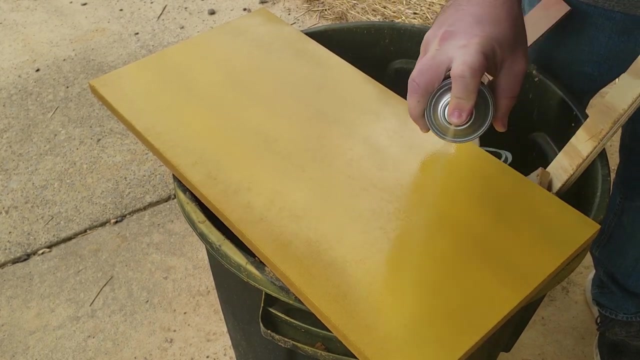 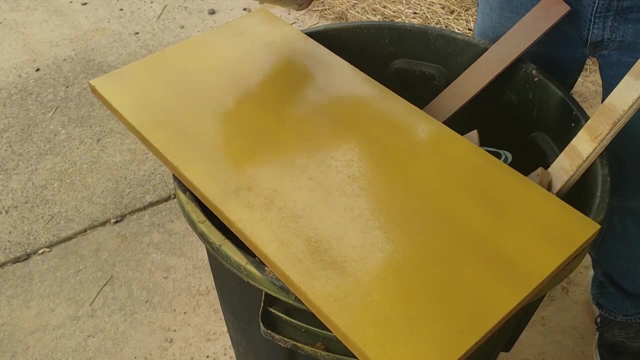 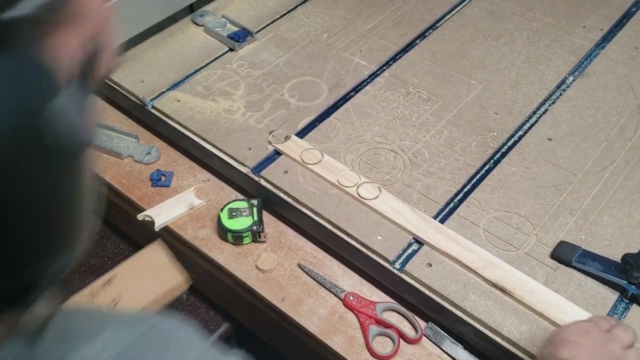 Now I'll be putting the sides together. Using some spray paint I had on hand, I painted the base and the side rails. MDF will be really rough after your first coat of paint, so it's important to sand it between coats. I'm using my CNC here, but this is way overkill. 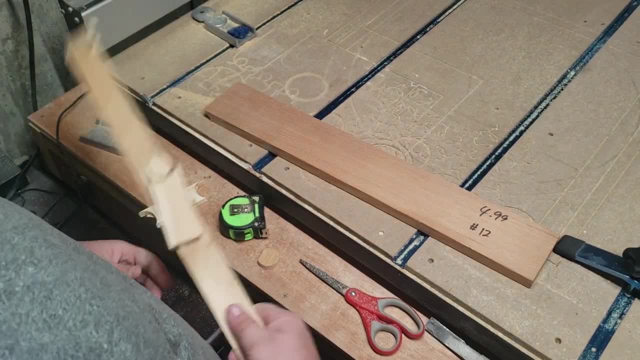 You could easily just buy a 1 inch dowel from your home goods store and cut it down to size for pucks. I'm using my CNC here, but this is way overkill. You could easily just buy a 1 inch dowel from your home goods store and cut it down to size for pucks. I'm using my CNC here, but this is way overkill. You could easily just buy a 1 inch dowel from your home goods store and cut it down to size for pucks. I'm using my CNC here, but this is way overkill. 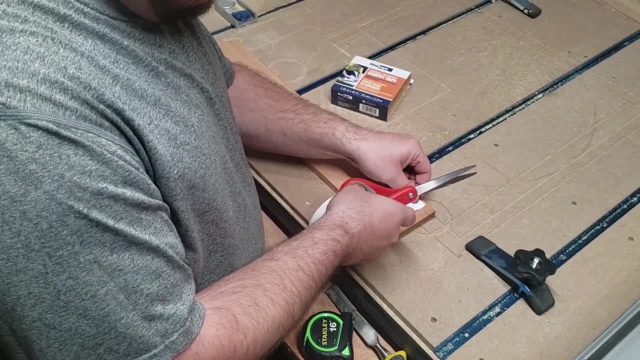 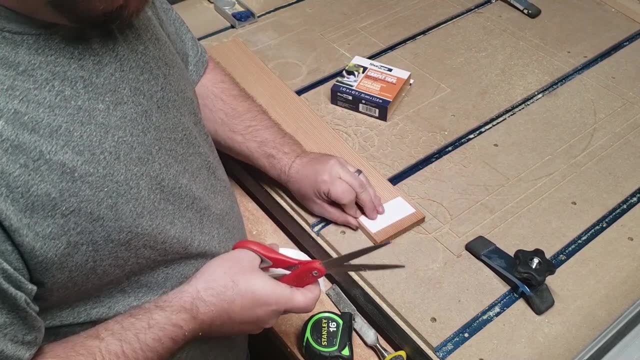 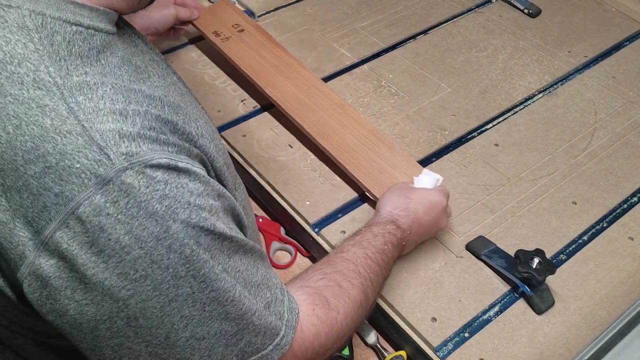 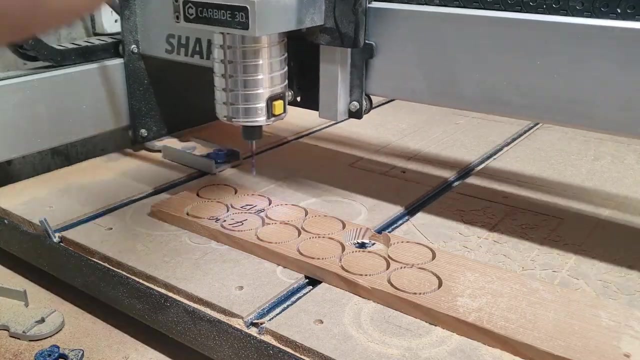 You could easily just buy a 1 inch dowel from your home goods store and cut it down to size for pucks. I'm using my CNC here, but this is way overkill. I'm using my CNC here, but this is way overkill. 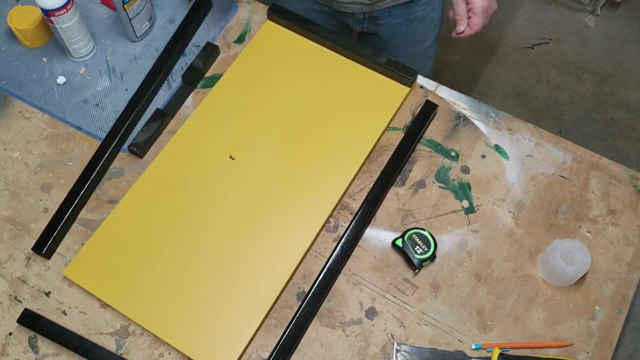 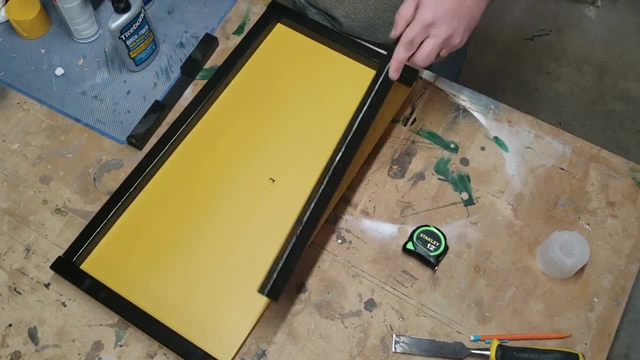 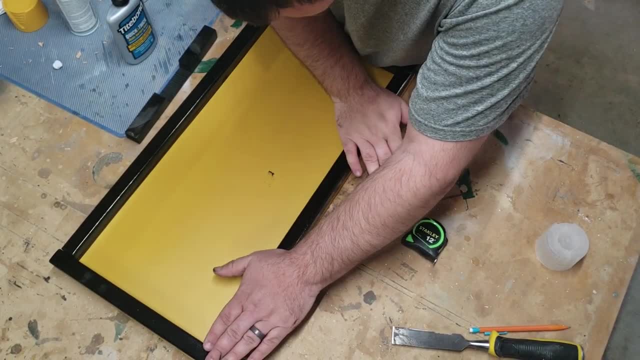 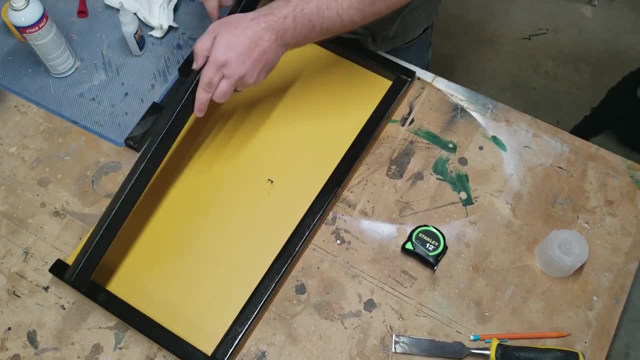 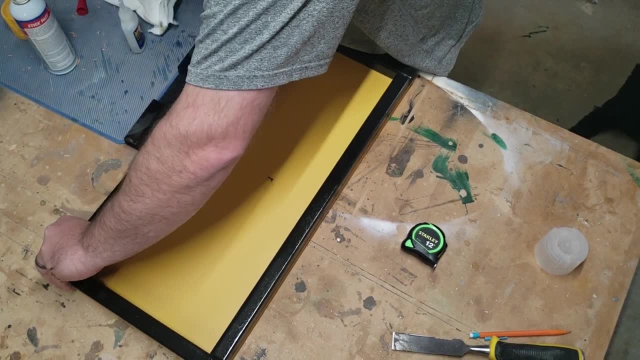 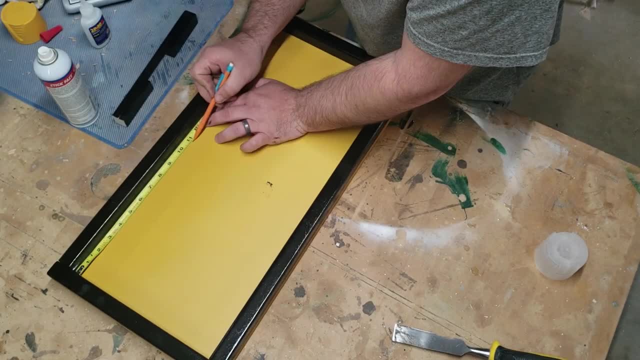 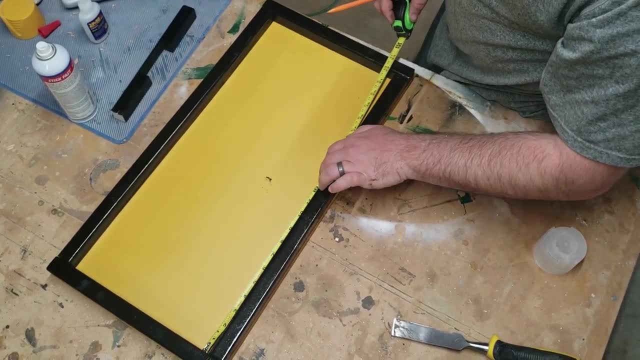 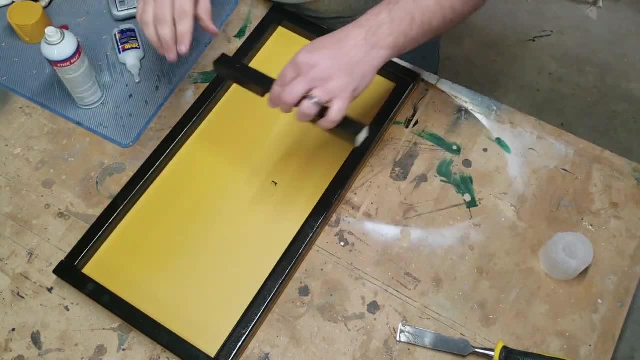 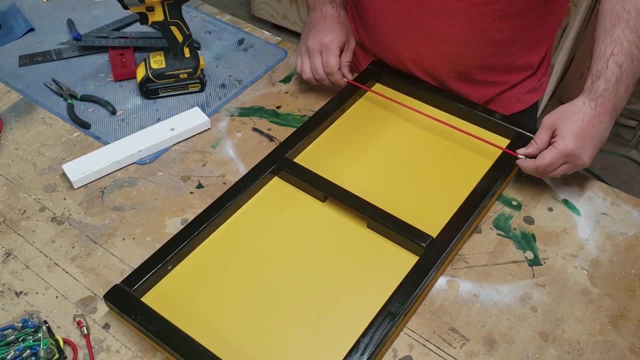 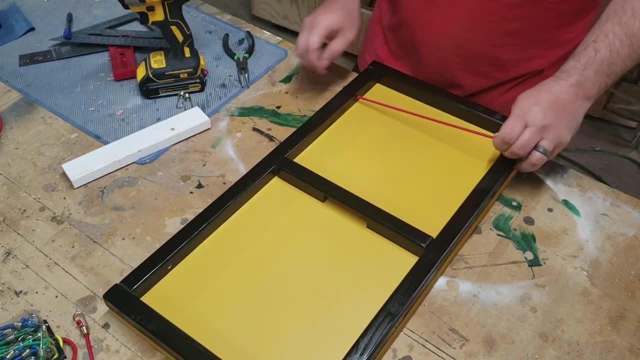 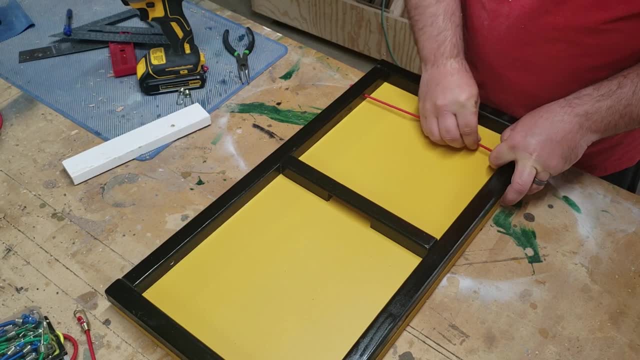 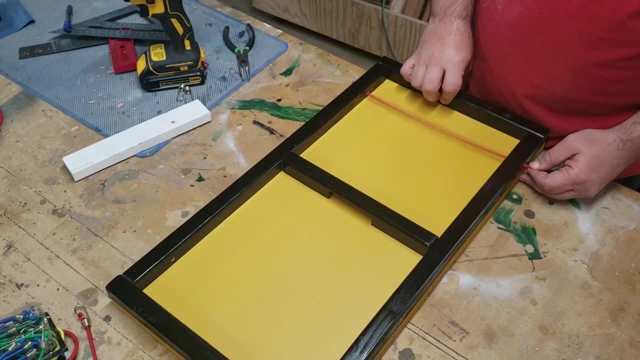 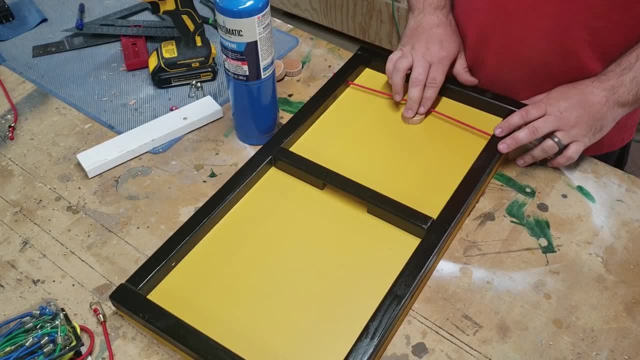 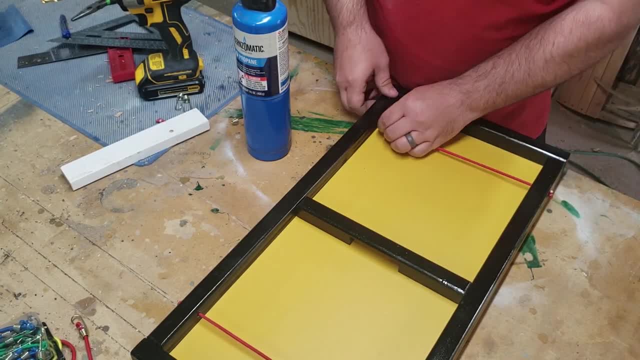 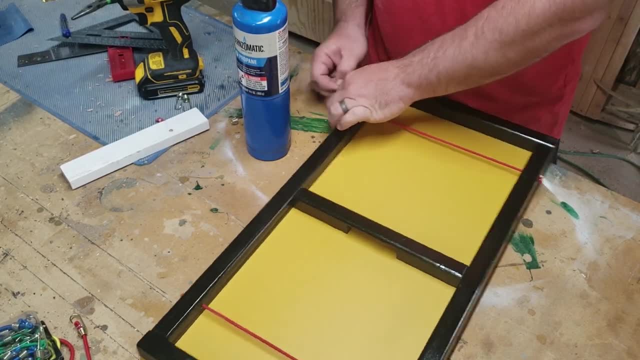 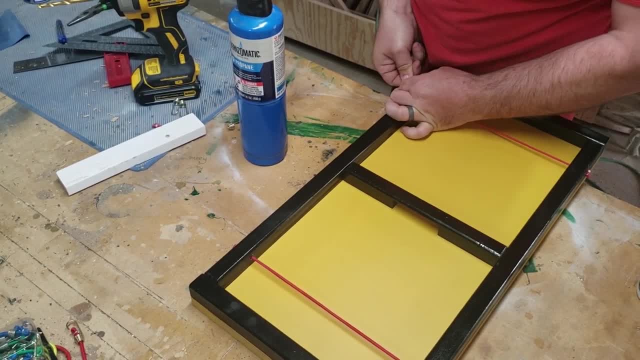 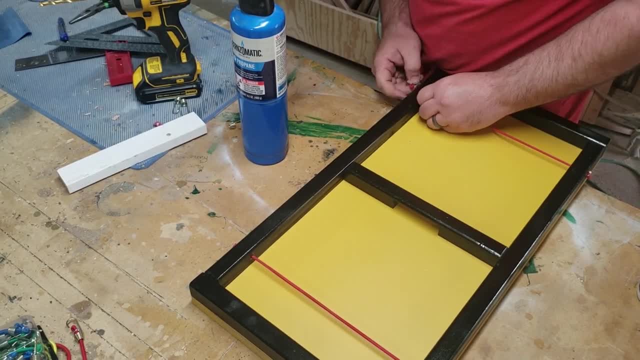 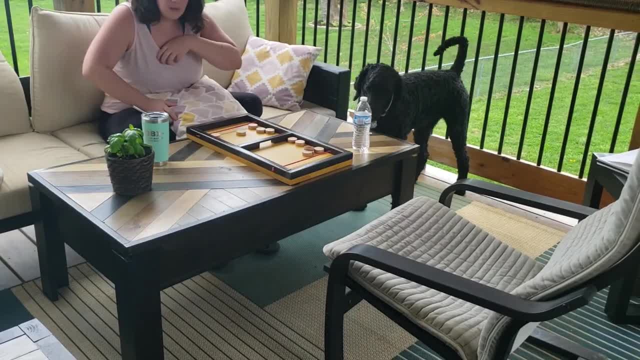 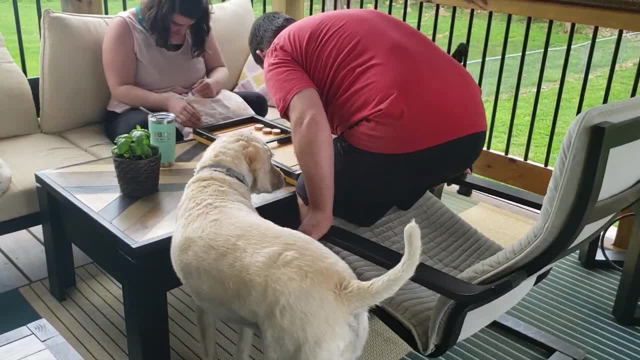 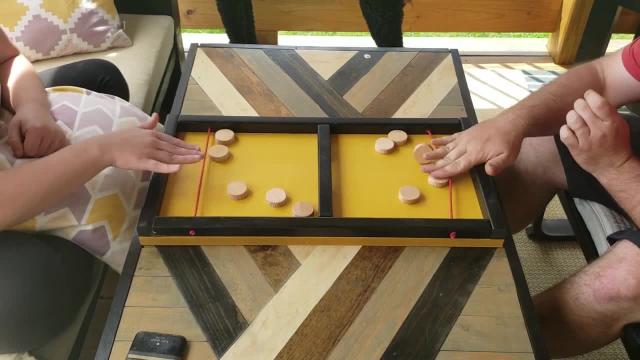 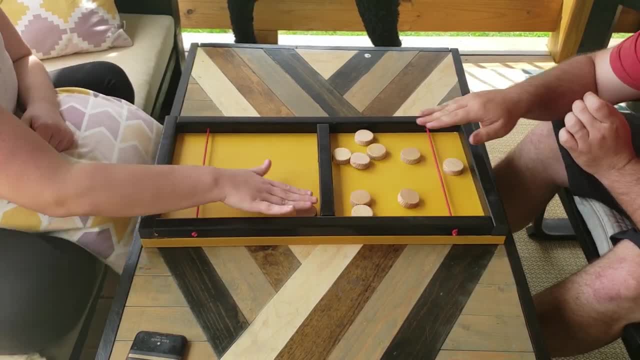 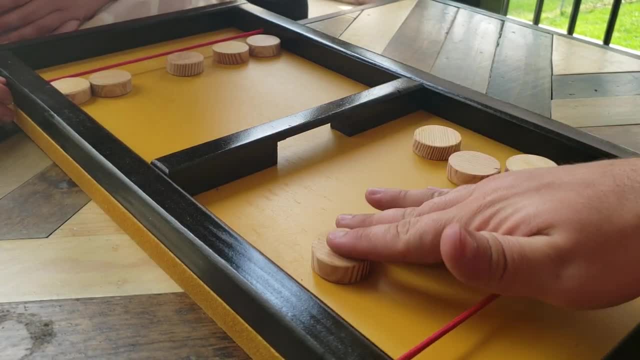 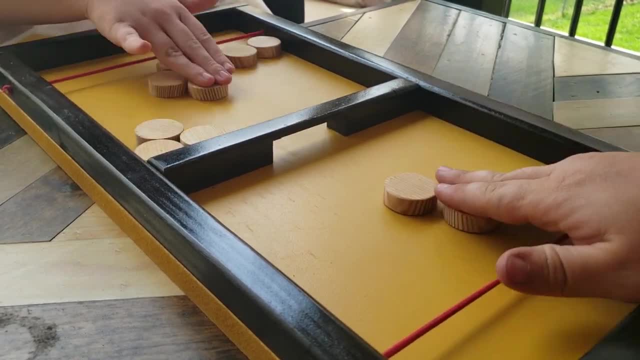 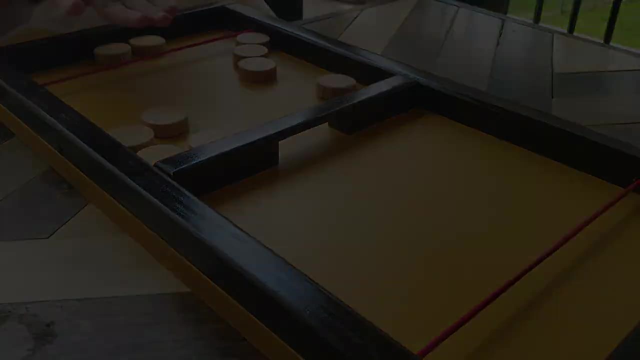